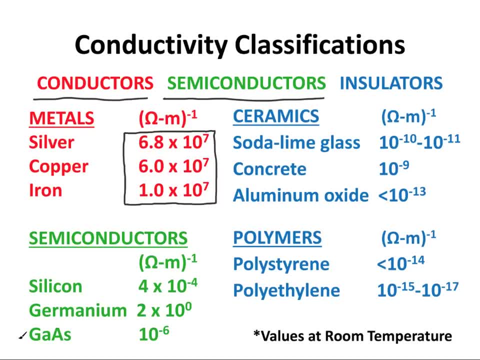 or they can be compound semiconductors that contain a group 3 and group 5 element. like gallium arsenide Semiconductors have a range of about 10 to the 0th power and they have a conductivity range of about 10 to the 9th power to 10 to the negative 6th power. 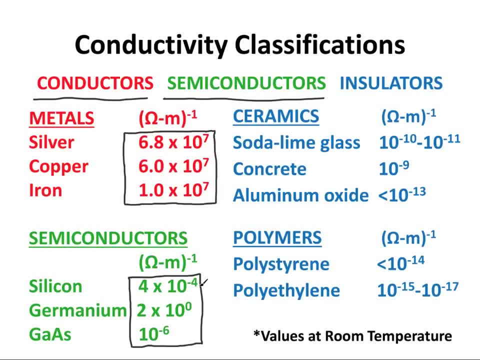 inverse ohm inverse meter, which is about 10 orders of magnitude less than the conductivity of metals. This means that they have a moderate conductivity. Insulators consist of ceramics and polymers and they have a low conductivity range of anywhere from 10 to the negative 9th power to ten to the negative 17th power. inverse ohm inverse meter. 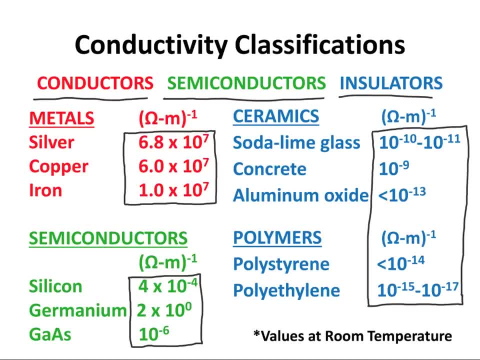 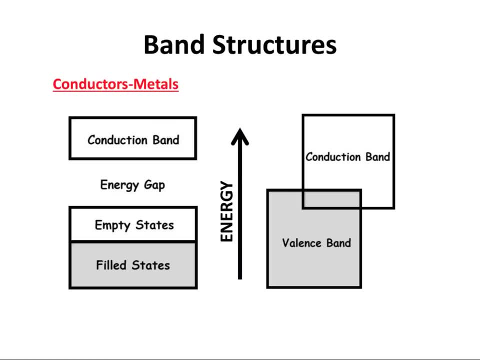 which is about 20 orders of magnitude less than the conductivity of metals. So why do conductors, semiconductors and insulators have such different levels of conductivity? To begin to understand these differences in conductivity, we first need to talk about band structures. 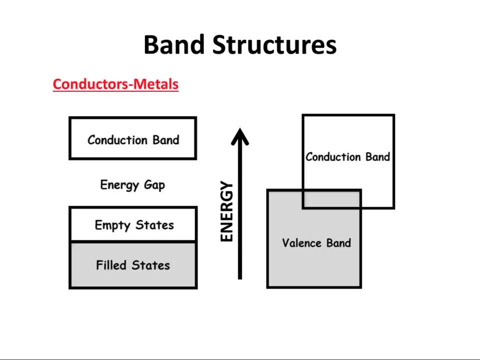 Band structures are related to the electronic energy states of a material. For metals, there are two potential band structure types, The first one being we have a half-full valence band followed by an energy gap, and then the conduction band. Electrons will move from the filled states to the empty states, because the higher energy levels of the empty states are easily accessible to these electrons. 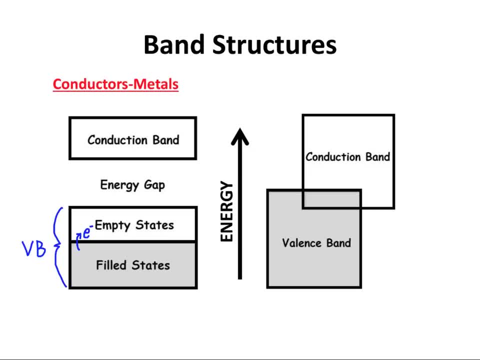 A good example of a metal with the half-full valence band would be sodium. Sodium has an electron configuration that ends in 3s1.. So one of two electrons are occupying the valence band. Sodium has a conductivity of about 2.1 times 1.. 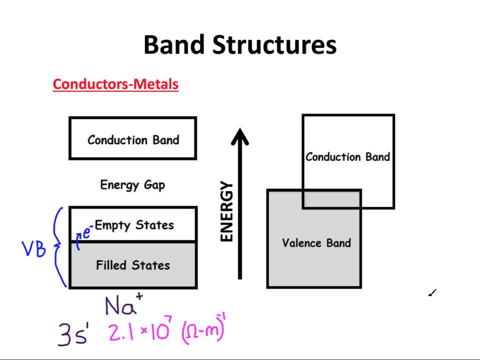 Sodium is 10 to the 7th power inverse ohm inverse meter. The other type of band structure for metals would be the overlapping band structure, where we have the valence band and the conduction band. overlapping Electrons will move from the valence band to the empty conduction band because, again, these higher energy levels are easily accessible to these electrons. 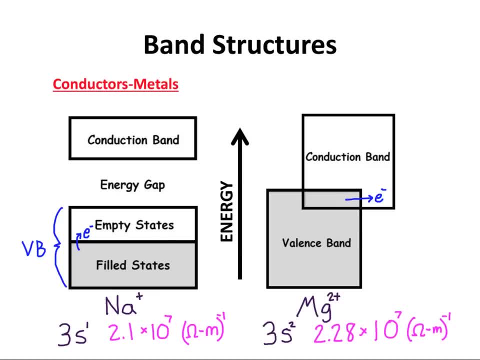 A good example of the overlapping band structure would be magnesium. Magnesium has an electron configuration that ends in 3s2.. So two out of two electrons occupy the valence band. It has a conductivity of about 2.28 times 10 to the 7th power. inverse ohm. inverse meter. 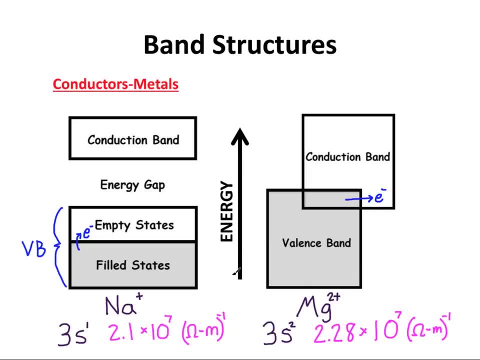 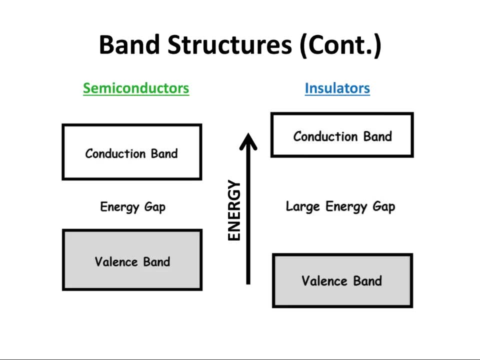 For metals. all atoms contribute their valence electrons to the conduction. So from these examples we can see that metals have high conductivity values. The band structure for semiconductors has a full valence band followed by an energy gap. A forbidden energy states that the valence electrons will move to the empty states. 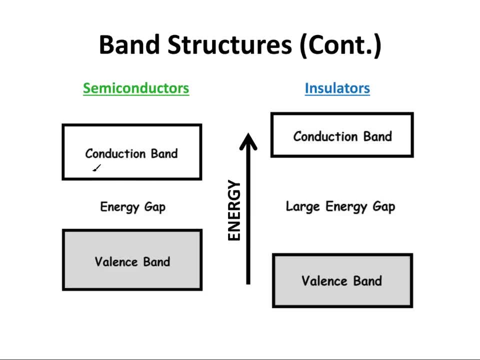 This means that the valence electrons can't occupy, followed by an empty conduction band. At a temperature of absolute zero, the conduction band is empty. Increasing the temperature provides the energy for electrons to jump from the valence band into the conduction band and leave behind an electron hole. 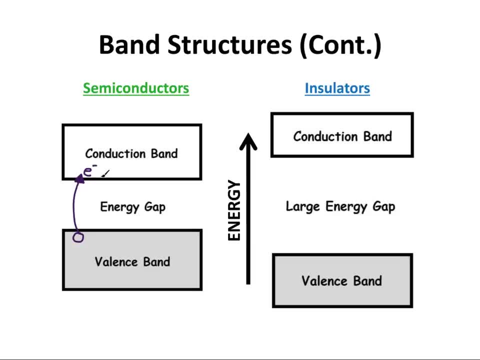 This is often referred to as an electron hole pair. The energy gap size for semiconductors is usually between 0.1 and 2 electrons. A good example for an intrinsic semiconductor might be silicon. Silicon has an energy gap of 1.12 electron volts and a conductivity of 4 times 10 to the negative 4th inverse ohm inverse meter. 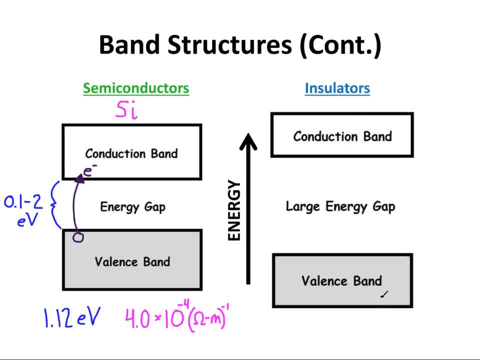 Insulators have a full valence band followed by a large energy gap which consists of forbidden energy states that the valence electrons cannot occupy. This means that the valence electrons can't occupy, followed by an empty conduction band. Again, at a temperature of absolute zero, there are no electrons in the conduction band. 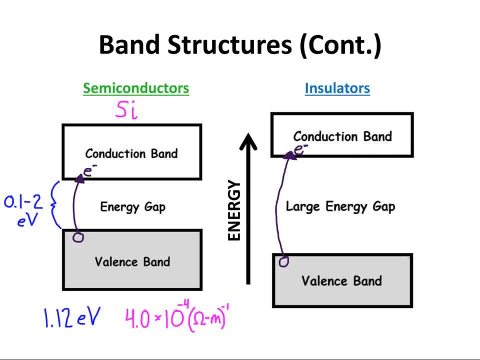 But with thermal energy the electron will jump from the valence band to the conduction band and create an electron hole pair. However, the energy gap size for insulators is somewhere between 2 and 6 electron volts, so it's much larger than semiconductors. 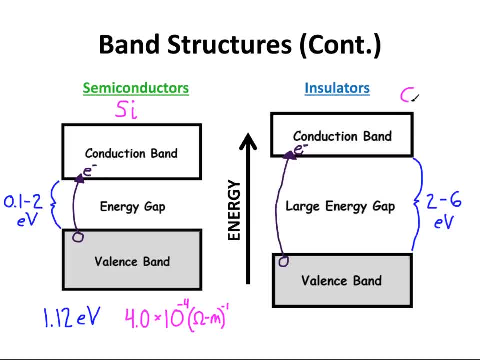 A good example for an insulator might be silicon. A good example for an insulator might be carbon in its diamond form. Carbon in its diamond form has an energy gap of 5.5 electron volts and a conductivity around 10 to the negative 17th power. inverse ohm. inverse meter. 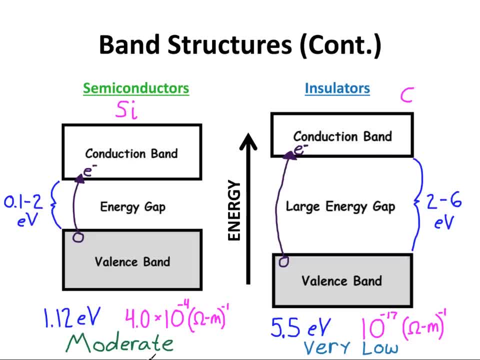 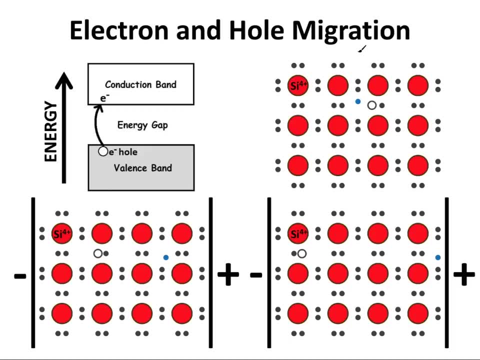 From these values we see that semiconductors have a moderate conductivity, while insulators have a very low conductivity. The next topic is electron and electron hole migration within semiconductors such as intrinsic silicon, As discussed in the previous slide, electron hole pairs are created by thermal energy when an electron is able to jump the energy gap into the conduction band. 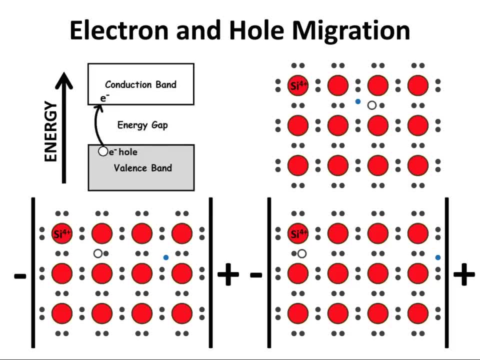 As shown here. in the first picture we can see this electron hole pair here. Now we have an empty bound state and we have a free electron created by thermal energy being provided to the semiconductor. In the next picture we see that we have applied a negative and positive bias. 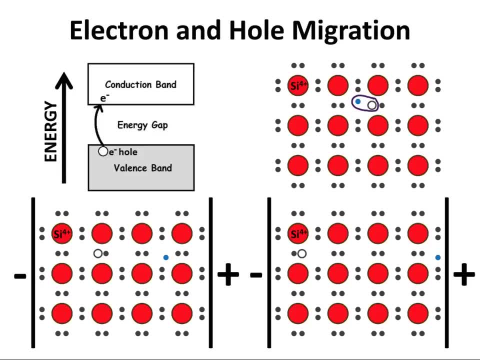 Otherwise known as an electric field, And we see that the electron hole will migrate towards the negative bias by an electron jumping into this available bound state. This is why electron holes are referred to as positive charge carriers, because they move towards the negative bias during the migration. 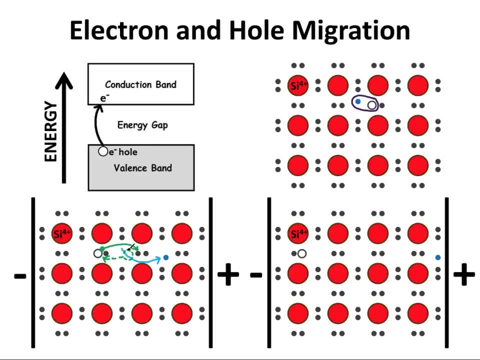 Simultaneously we have the free electron, which will move towards the positive bias because electrons are negative charge carriers. In the third picture we see that again the hole will move even further towards the negative bias by an electron jumping into the available bound state. 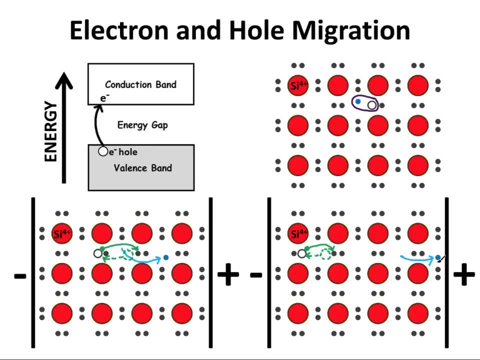 And the free electron is going to move even closer to the positive bias. The free electron moves more easily in the conduction band than the electron hole moves in the valence band. So the mobility of the free electron is higher than the mobility of the electron. 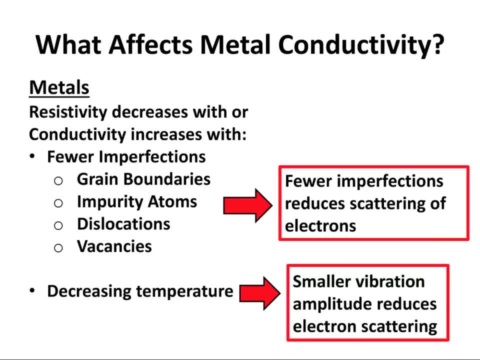 So the mobility of the free electron is higher than the mobility of the electron hole during migration. We've already discussed the two types of metal band structures that are used to represent the energy states of the valence electrons. Now we're going to discuss what factors affect the conductivity of metals. 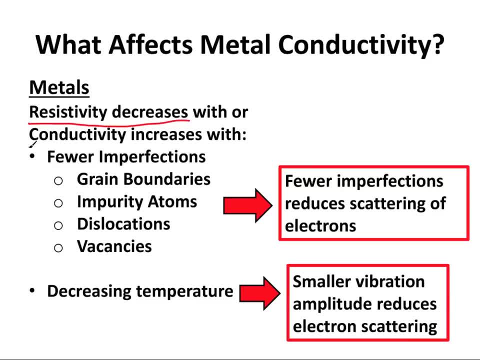 For metals, resistivity decreases with, or conductivity increases with, fewer imperfections. Imperfections such as grain boundaries, impurity, atoms dislocations and vacancies scatter electrons. So when we have fewer imperfections, we reduce the scattering of electrons and increase the conductivity. 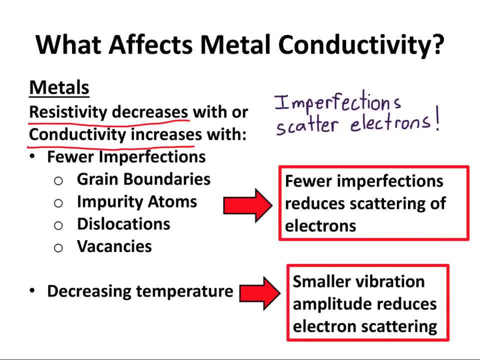 Imperfections, such as dislocations and vacancies, can be reduced by having less cold work. So if you have an annealed copper bar and a cold work copper bar, the annealed copper bar will have a higher conductivity because it has less cold work. another way to increase the conductivity would be to decrease the temperature. 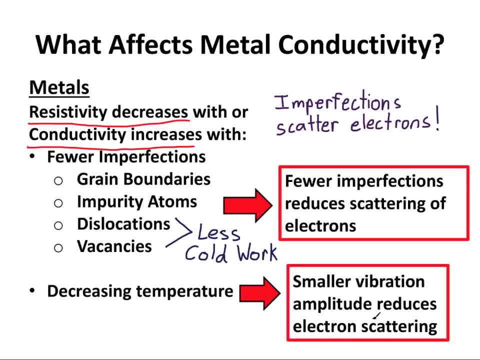 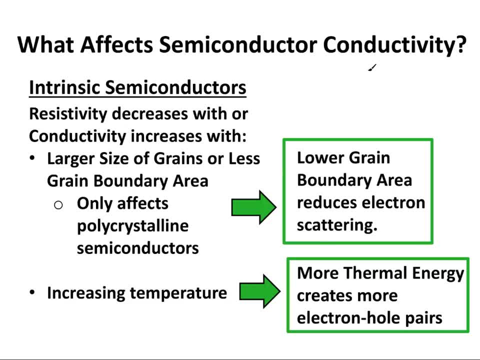 By decreasing the temperature we have smaller atomic vibration amplitude, which reduces electron scattering. So what factors affect the conductivity of semiconductors? For intrinsic semiconductors, resistivity decreases with, or conductivity increases with, larger size of grains or less grain boundary area. 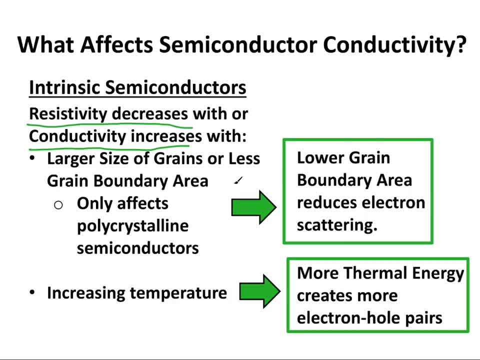 Grain boundary area is an imperfection in semiconductors That scatters electrons. So when we have lower grain boundary area, we reduce the electron scattering. This is only relevant for polycrystalline semiconductors. Another factor that affects the conductivity of semiconductors would be temperature. 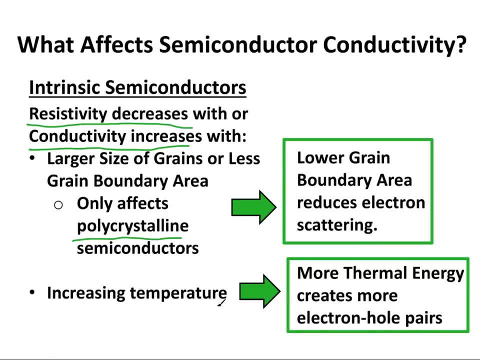 By increasing the temperature we increase the conductivity of the semiconductor because more thermal energy creates more electron hole pairs. So insulators create electron hole pairs through thermal energy. So if we increase the temperature of insulators we provide more thermal energy and therefore we have more electron hole pairs, which increases the conductivity. 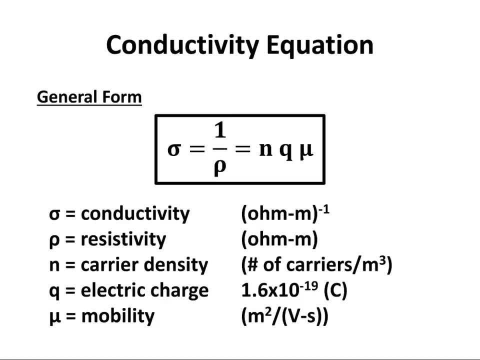 Since we have now addressed the basic concepts of electronic properties of materials, we can discuss the conductivity equation and how it is applied to each type of material. In its general form, we have that the conductivity is equal to the inverse of resistivity. So, while the units for resistivity are omega, 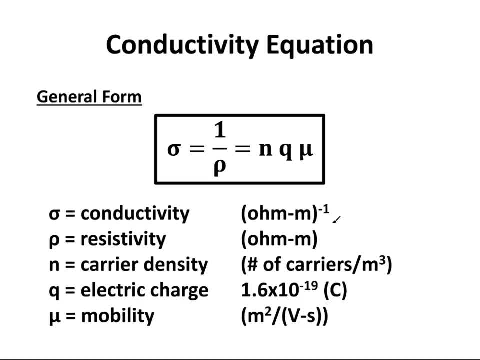 the units for conductivity will be inverse, ohm, inverse meter. To calculate this conductivity, there are three main terms. We have the carrier density, otherwise referred to the number of charge carriers per meter cubed of the material multiplied by the electric charge constant. 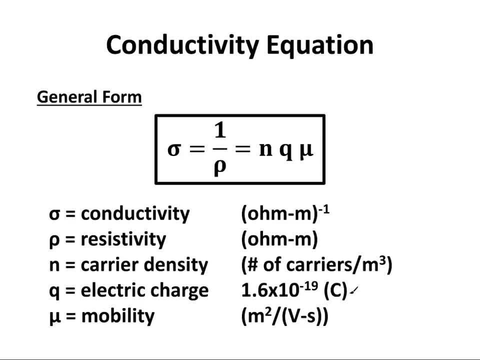 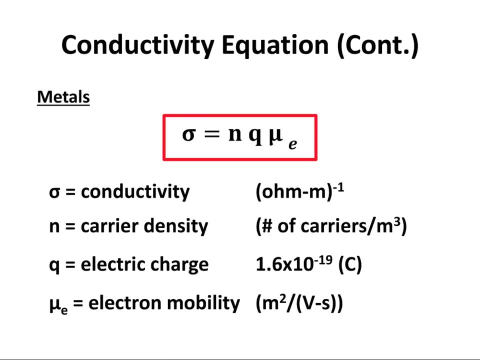 which is always 1.6 times 10 to the negative 19th power coulombs. And then, finally, we have the mobility of our charge carriers, And the units for that are meter squared per volt second, because mobility will only occur when we have an electric field applied. 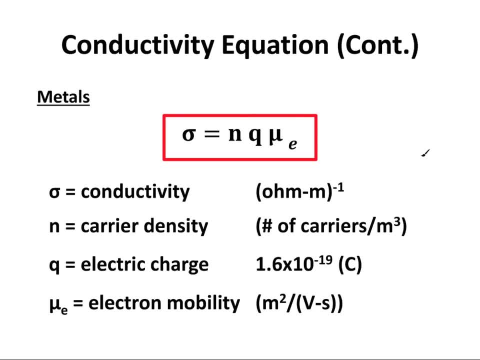 When we apply the conductivity equation to metals, we have: the conductivity equals the charge carrier density or number of carriers per meter cubed, multiplied by the electric charge constant 1.6 times 10 to the negative 19th power coulombs. 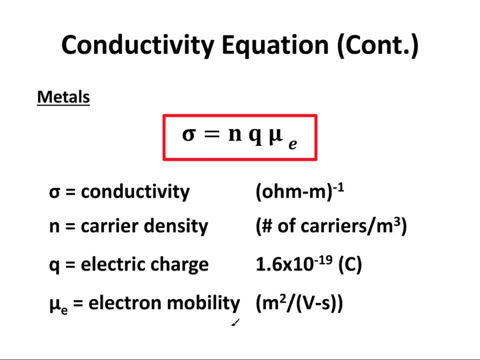 and multiplied by the electron mobility. For metals, conductivity is due to the valence electrons. Every atom contributes its valence electrons to the conductivity which we have referred to as a sea of electrons in the bonding. So that's why we use electron mobility in the conductivity equation. 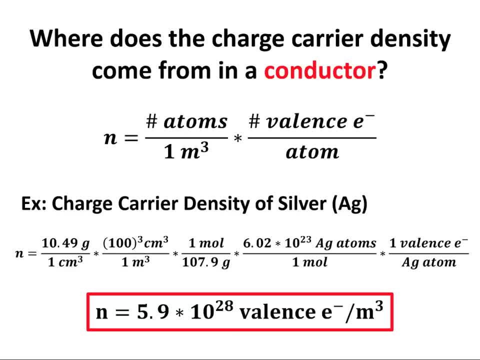 So where does the charge carrier density come from in a conductor? The charge carrier density of a conductor is going to be equal to the number of atoms per meter cubed multiplied by the number of valence electrons per atom. This is because every atom in the material 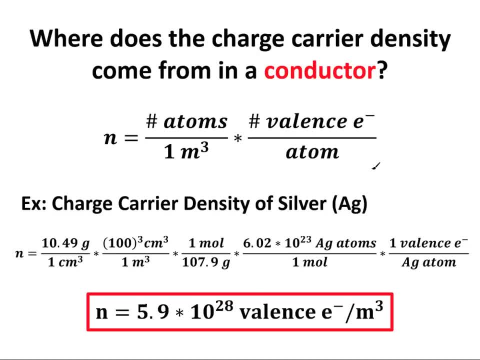 is going to contribute its valence electrons towards conductivity. For example, we're going to calculate the charge carrier density of silver. Normally we do not know how many atoms are in one meter cubed of a material, but we usually know the density of the material. 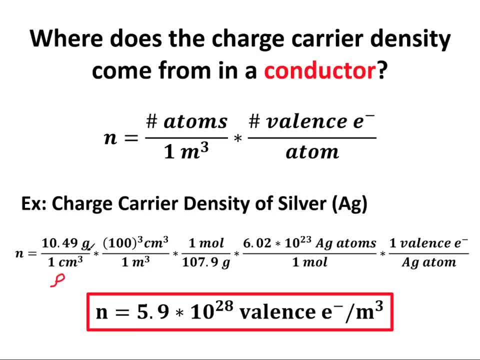 The density of silver is 10.49 grams per centimeter cubed. So we're going to use dimensionality, We're going to use dimensional analysis in order to get from density to the number of atoms per meter cubed. First we multiply by 100 to the third power: centimeters cubed per meter cubed. 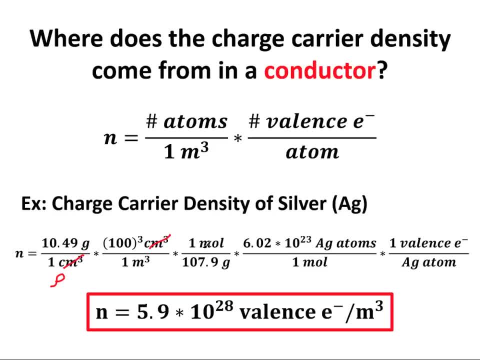 in order to cancel out the centimeter cubed units, Then we multiply by one mole divided by 107.9 grams, or the molar mass of silver, such that the grams cancel out. Then we multiply by Avogadro's number. 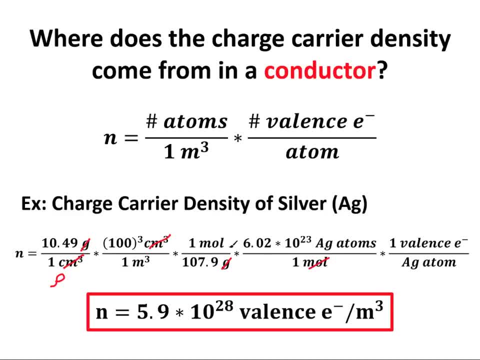 which is the number of silver atoms per one mole, such that the mole units here cancel out. As you can see what we're left with for units, we have the number of silver atoms per meter cubed, The final step to find the carrier density of silver. 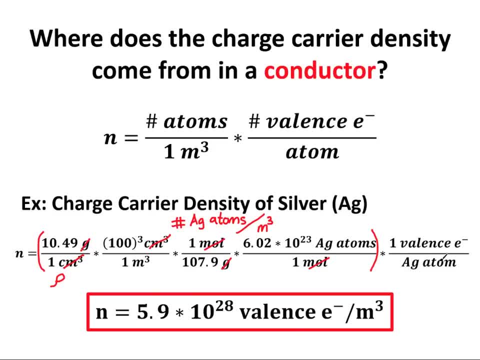 is going to be multiplying this number by one valence electron per silver atom, Finishing the calculation, we see that the carrier density of silver is 5.9 times 10 to the 28th power valence electrons or charge carriers per meter cubed. 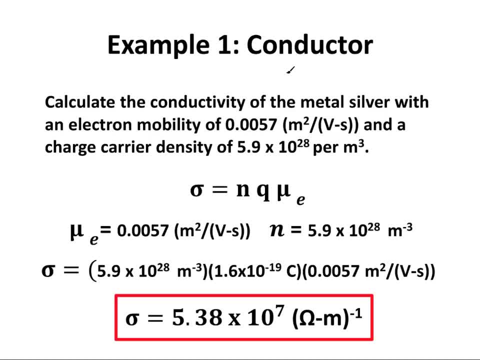 For example 1, we will be calculating the conductivity of a conductor. Calculate the conductivity of the metal silver with an electron mobility of 0.0057 meters squared per volt second and a charge carrier density of 5.9 times 10 to the 28th power per meter cubed. 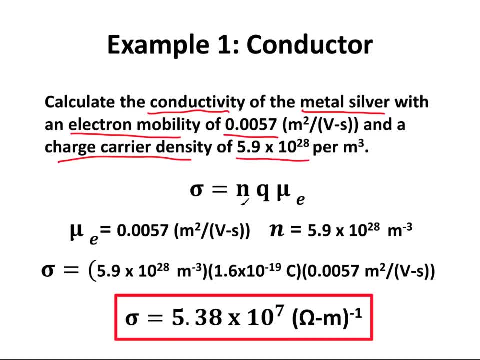 Since we have a metal like silver, we need to use the conductivity equation for conductors, which is the conductivity equals charge carrier density times the electric charge constant Q multiplied by the electron mobility. In the problem, we were given these values for the electron mobility. 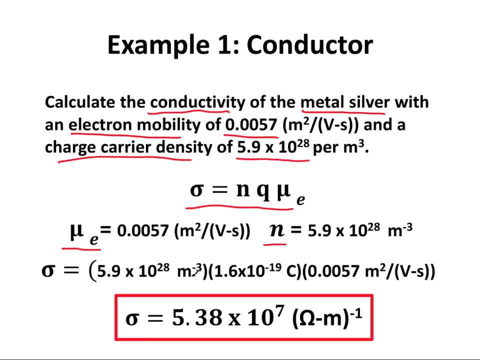 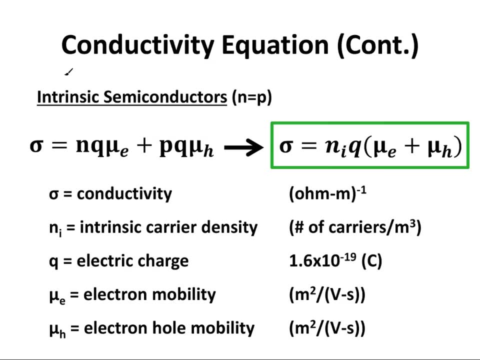 and for the charge carrier density, such that when we plug these values in to the conductivity equation along with the electric charge constant, we get a conductivity of 5.38 times 10 to the 7th power inverse ohm inverse meter. Now we're going to talk about the application of the conductivity equation. 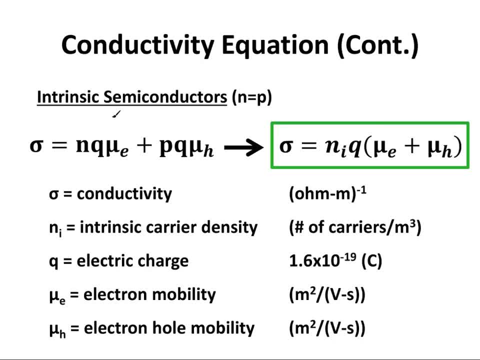 to semiconductors. For intrinsic semiconductors we have two contributions to the conductivity equation. The first contribution is due to the electrons and the second contribution is due to the electron holes. The electrons contribute conductivity by the number of negative charge carriers. 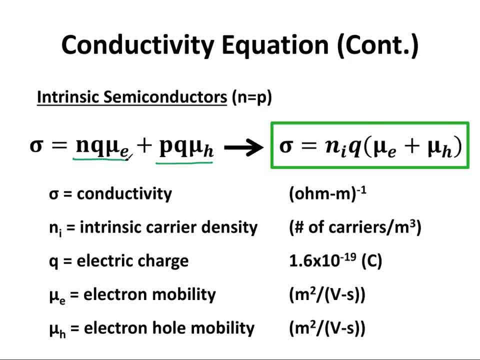 multiplied by the electric charge constant, multiplied by electron mobility. Then for the positive charge carriers, or the electron holes, we would multiply by the electric charge constant and by the mobility of those electron holes. So for intrinsic semiconductors we have electron hole pairs. 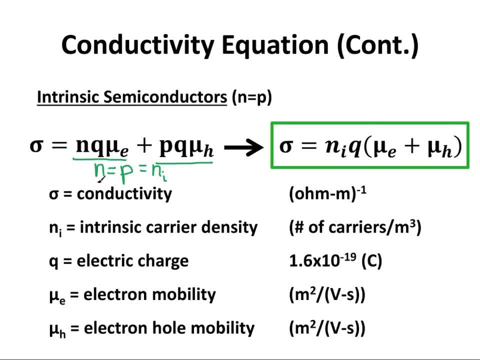 Therefore, we can say that the number of negative charge carriers is equal to the number of positive charge carriers, which we then refer to as the intrinsic carrier density. We can simplify this conductivity equation to have the intrinsic carrier density multiplied by the electric charge constant. 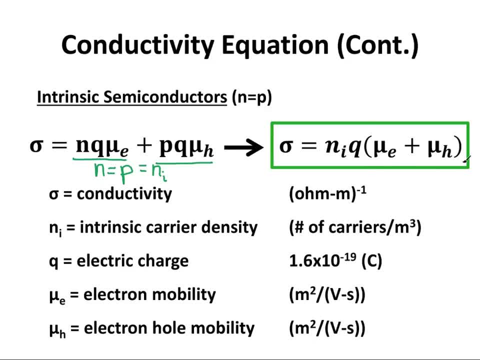 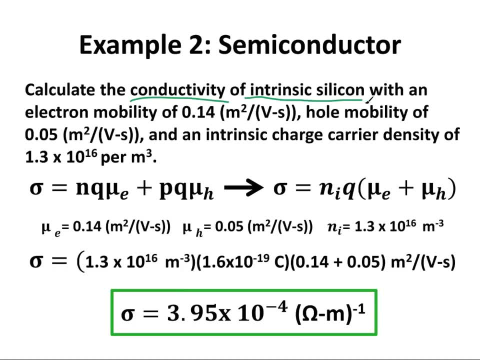 and then multiplied by the summation of the electron and hole mobilities, For example 2,, we need to calculate the conductivity of intrinsic silicon with an electron mobility of 0.14 meters squared per volt second hole mobility of 0.05 meters squared per volt second. 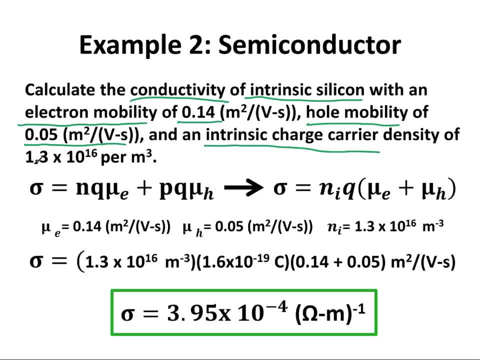 and an intrinsic charge carrier density of 1.3 times 10 to the 16th charge carriers per meter cubed. As discussed in the previous slide, the conductivity of semiconductors has both an electron contribution and an electron hole contribution. 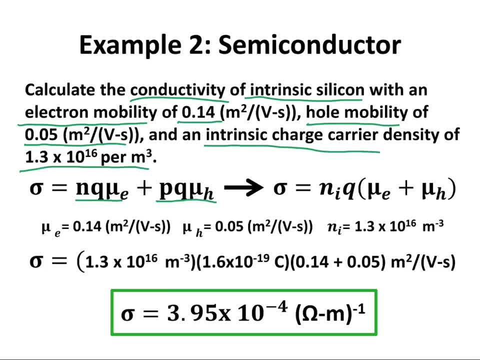 Because we were told it's intrinsic silicon. we can say that the number of negative charge carriers is equal to the number of positive charge carriers, which we call the intrinsic charge carrier density. Therefore, we can use the simplified form of the conductivity equation for semiconductors. 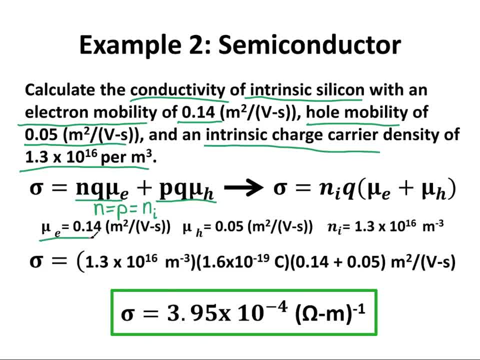 In the problem, we were told, the mobility of the electrons, the mobility of the holes and the intrinsic charge carrier density, such that when we enter them into the conductivity equation for semiconductors, we have that the conductivity of intrinsic silicon will be 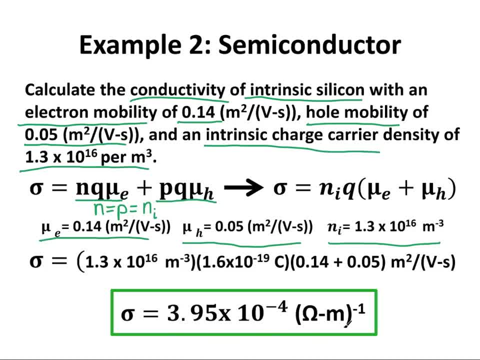 3.95 times 10 to the negative fourth power. inverse ohm inverse meter. An important note about the conductivity of semiconductors would be that the contribution of the electrons to conductivity is greater than that of the contribution by electron holes. The reason is that the mobility of electrons 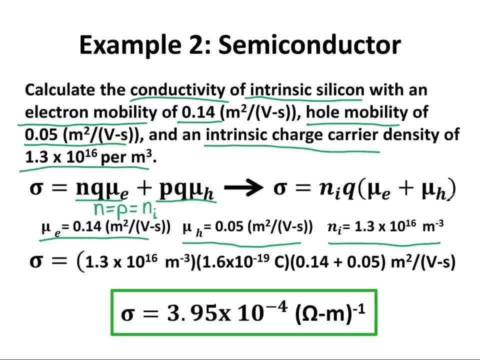 is usually much higher than the mobility of electron holes. In the case of silicon, we can see that the electron mobility is more than twice the amount of the mobility of the electron holes. So overall electrons contribute most of the conductivity for semiconductors. 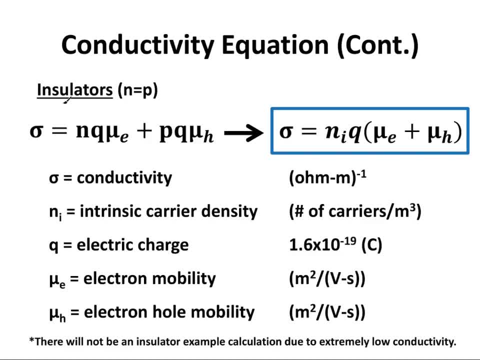 The conductivity equation for insulators is rather similar to that of semiconductors. Insulators have a conductivity contribution from both the electrons and from the electron holes. We have the negative charge carrier density multiplied by the electric charge constant, multiplied by the electron mobility. 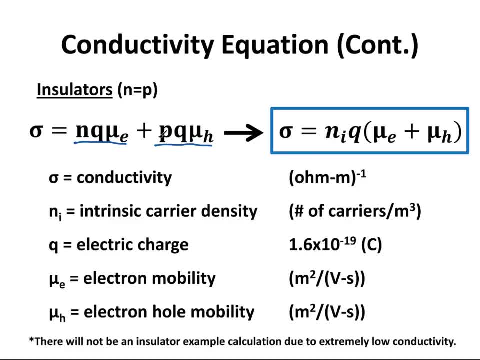 for the contribution of the electrons, For the contribution of the electron holes, we have the positive charge carrier density times the electric charge constant multiplied by the hole mobility. Because we have electron hole pairs, we say that the number of negative charge carriers is equal to the number of positive charge carriers. 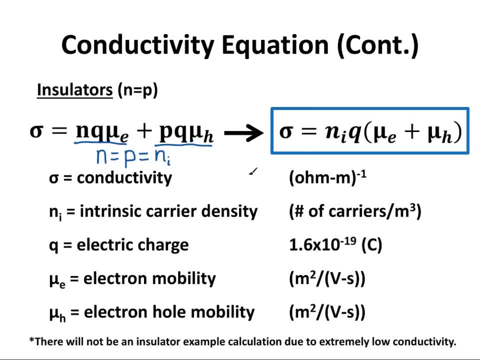 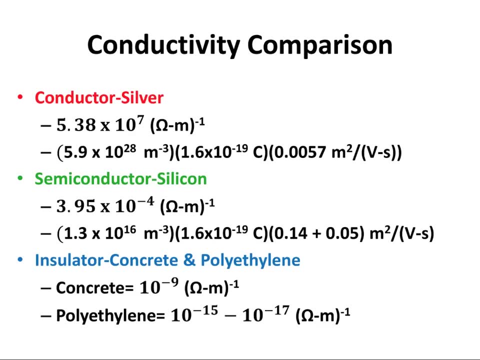 which we refer to as the intrinsic carrier density. So again we can simplify the conductivity equation for insulators to be the intrinsic carrier density multiplied by the electric charge constant and then multiplied by the summation of the electron mobility and the hole mobility. Now that we have discussed the band structures, 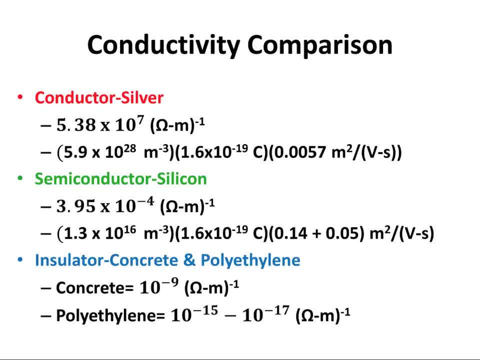 and conductivity equations for each type of electronic material. we can compare the relative differences that cause such varying levels of conductivity Using our examples for the conductor silver and the semiconductor silicon. the first thing we can recognize is that the mobility of the conductor silver is less than that of the mobility of the semiconductors. 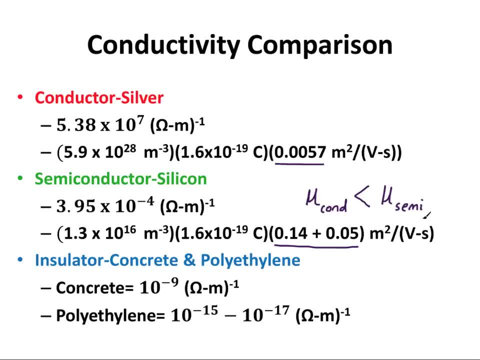 If the mobility of the conductors is less than the mobility of semiconductors, why do conductors have a higher conductivity than semiconductors? The answer lies with the carrier density. The carrier density of silver is along the order of magnitude of 10 to the 28th power. 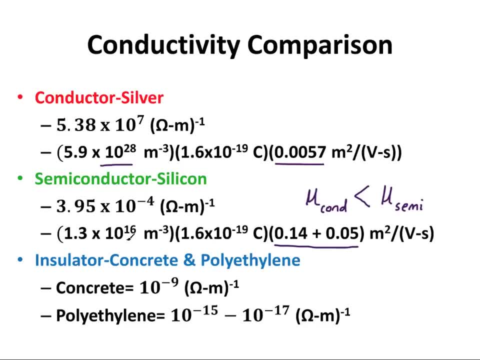 while the order of magnitude for the carrier density of silicon is about 10 to the 16th power. So in comparison, the carrier density of conductors is significantly greater than the carrier density of semiconductors. That's because every atom contributes all of its valence electrons. 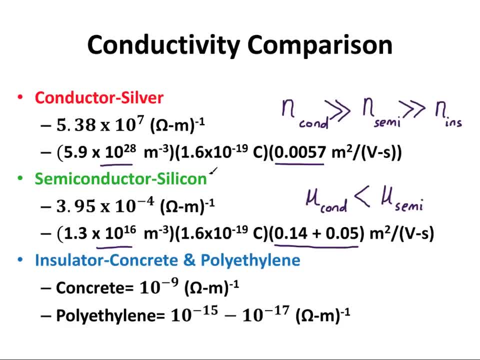 towards conductivity for conductors like silver, But in the case of a semiconductor like silicon, only a small fraction of the atoms can contribute electron-hole pairs through thermal energy, Bringing insulators into the picture. insulators have an even smaller carrier density than semiconductors. 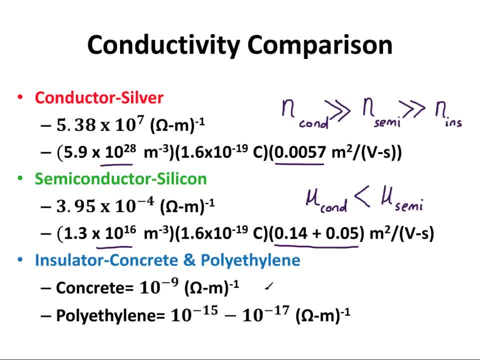 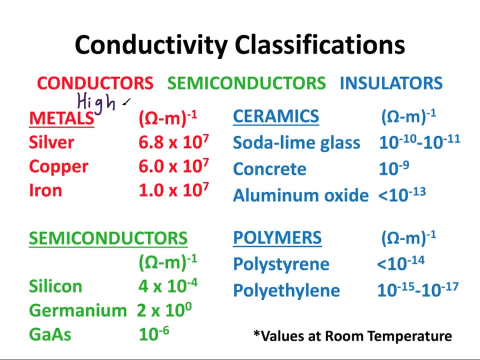 because an even lower fraction of atoms are able to contribute electron-hole pairs towards conductivity due to the increase of the energy gap in insulators. So, in summary, metals have a high conductivity because every atom contributes its valence electrons towards the conductivity of the metal. 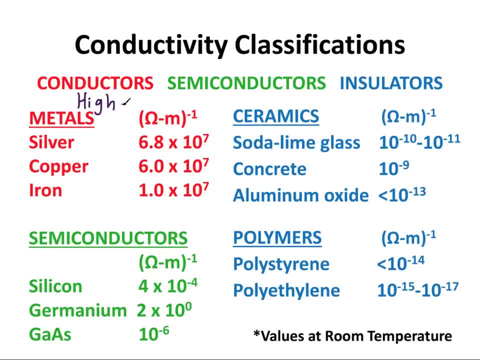 resulting in a very high carrier density For semiconductors. we may have a higher mobility in semiconductors than in metals, but the carrier density of semiconductors is significantly less than that of metals. only a small fraction of the atoms in semiconductors